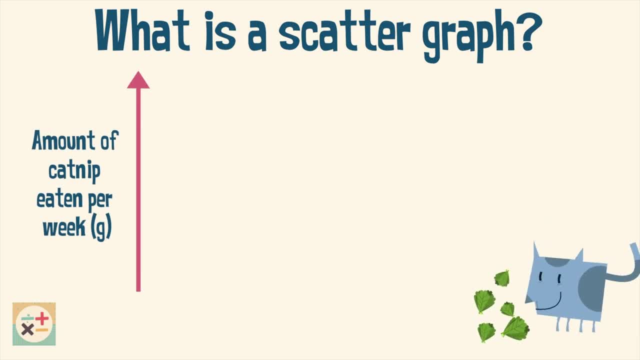 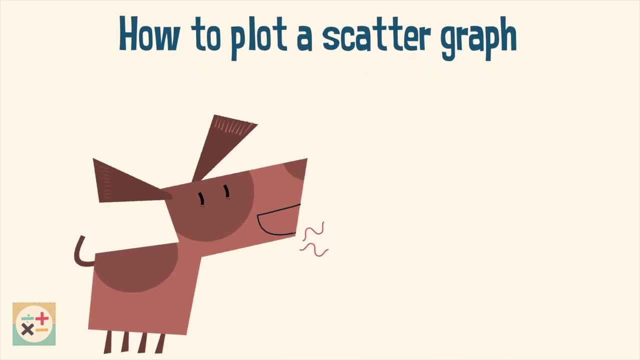 For example, it can show you if there is a relationship between the amount of catnip a cat eats and the length of its whiskers. So how do you plot a scatter graph? Have a look at this set of data. We are given values for the size of each dog in centimetres. 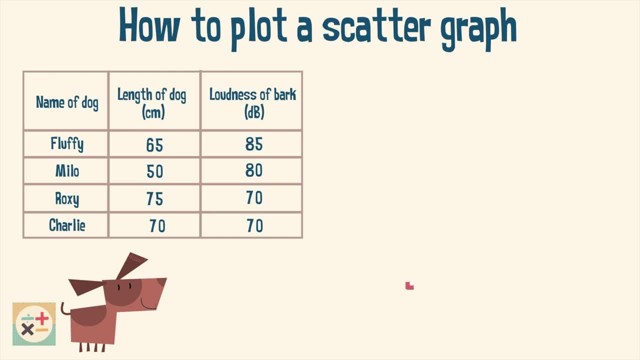 and the loudness of its bark in decibels. Let's first plot the values for the dog named Fluffy. Find 65 centimetres on the x-axis, labelled length of dog, and draw a line extending from this point. Then find 85 on the y-axis, labelled loudness of bark. 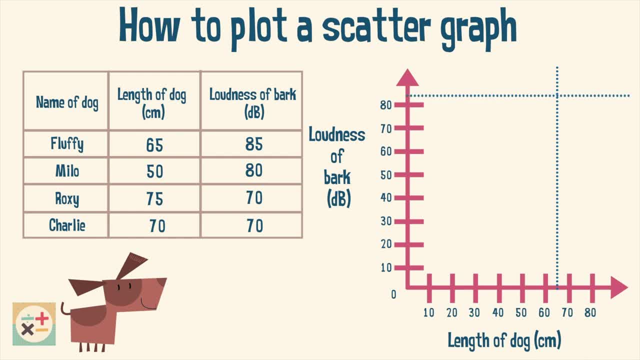 and draw a line extending from this. The point where the two lines cross is where we will draw the scatter plot. Now do the same for the other dogs. The scatter graph is now complete, Although this doesn't tell us much, as we would need data from more than four dogs to determine how the length of the dog 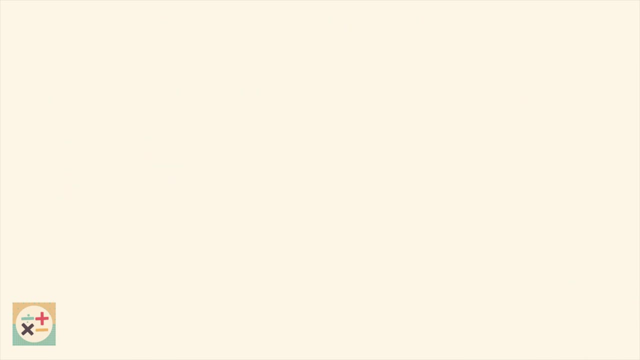 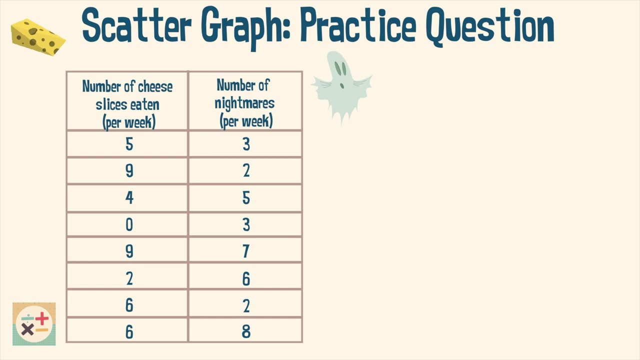 correlates to the loudness of its bark. Now have a go at this practice question. using the data provided and some graph paper, plot the points on a scatter graph. Pause the video while you do this. vested functions and low frequencies are available. 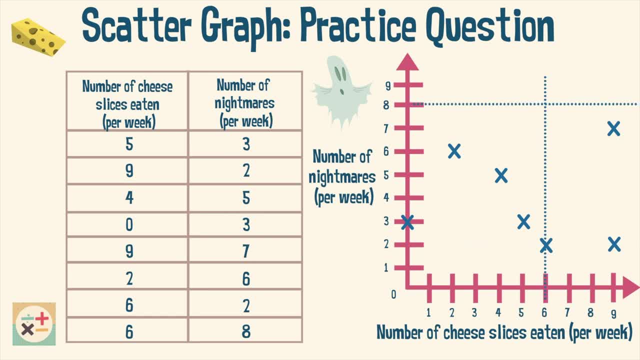 as well as additional digits, Three as necessary theüst. Thanks for watching Minity Maths. Check out the channel for more videos.